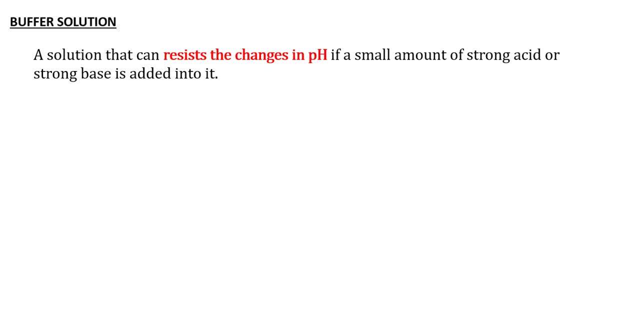 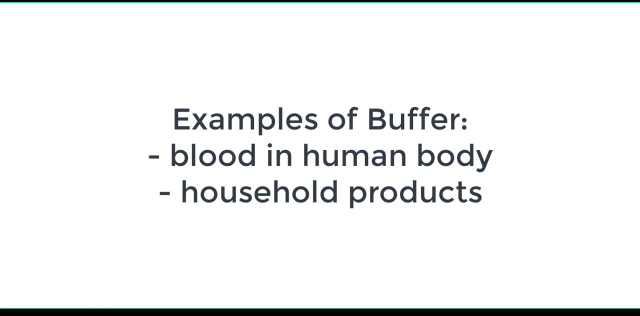 how much acid or base can be neutralized before the pH change. Examples of buffers are blood that contains a bicarbonate buffer system and also in many household products, For example, an adult shampoos are buffered to prevent the skin irritation by components like sodium. 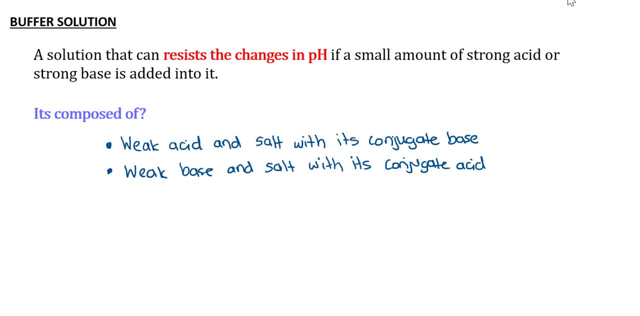 hydroxide. In order to maintain the pH range effectively, a buffer must consist of a weak conjugate acid-base pair, meaning either a weak acid and salt with its conjugate base or a weak base and salt with its conjugate acid. A buffer is able to resist the pH change because of the two components, which is the 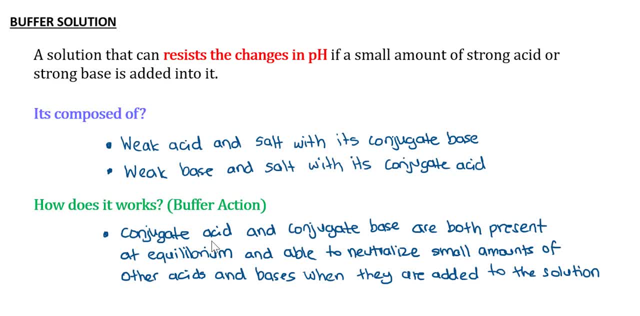 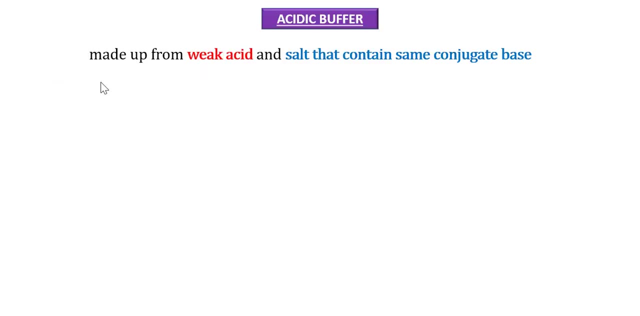 conjugate acid and conjugate bases that are both present at equilibrium and are able to neutralize the small amount of the other acid and base when they are added into a solution. To clarify this effect, we will discuss it later- An acidic buffer is a solution that is made up of a weak acid and salt that contains the 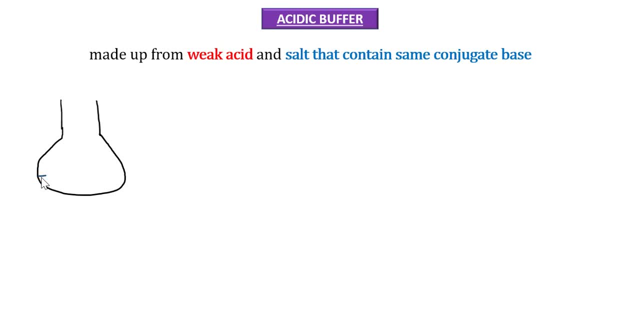 same conjugate base. This occurs when nada and kerosene are added to a solution and their base. for example, if we have a weak acid, which is an acetic acid, that are mixed with a sodium acetate salt, the sodium acetate salt will dissociate completely. 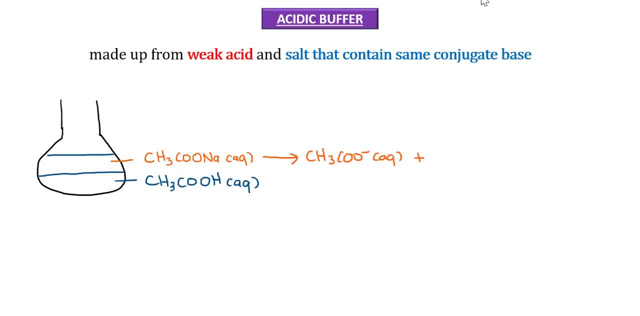 in water to form the acetate ion and also the sodium ion, while the acetic acid is a weak acid which will dissociate very slightly in water to form an acetate ion and hydronium ion. since this weak acid and salt contains the same conjugate base, this solution is a buffer solution. the conjugate base. 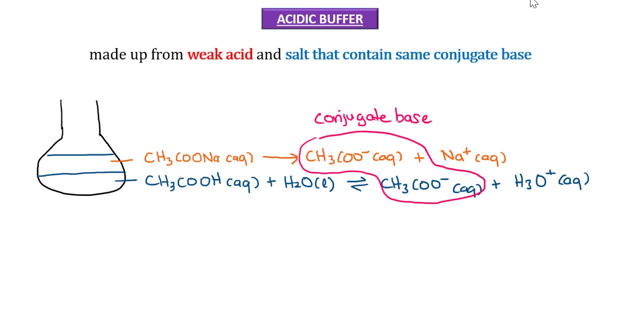 will become a basic species, while the weak acid will become an acidic species. you calculate the pH of the acidic buffer solution. we are going to use the Henderson-Hasselbalch formula, which is: pH is equals to pKa plus log concentration of conjugate base over concentration of a weak acid. remember pKa is equals to. 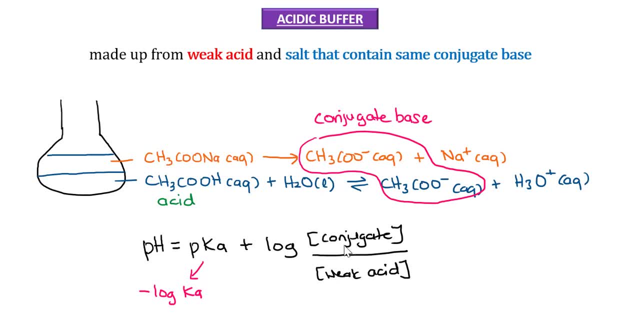 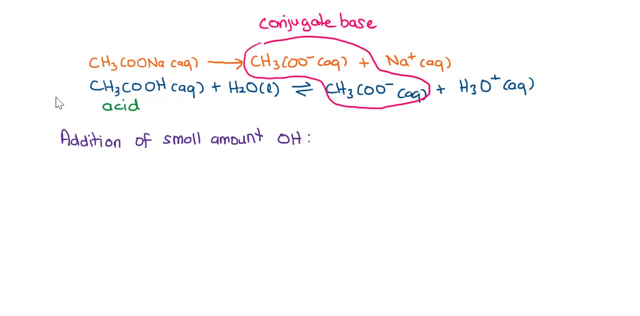 negative log Ka. the concentration of the conjugate base equals to the concentration of pKa. number z must be equal to the concentration of the salt, since the salt will fully dissociates and form the conjugate base ion. when a small amount of strong base is added in to the solution, weak acid will. 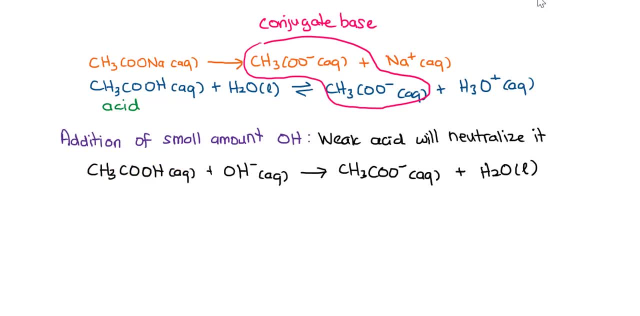 neutralize it. the weak acid will donate its proton to the base and from the conjugate base. this will make the concentration of the conjugate base. The equilibrium position will shift to the left to increase the concentration of the weak acid. Thus the pH is not much affected. 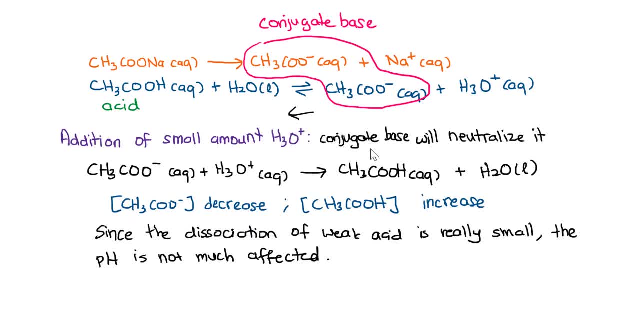 When a small amount of strong acid is added, a conjugate base will neutralize it. Thus, the concentration of the conjugate base will decrease and the concentration of weak acid increases. Since the dissociation of the weak acid is really really small, the pH is not much affected. 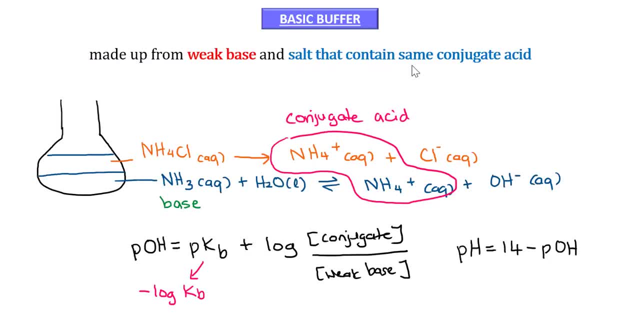 Basic buffer solution is made up from the weak base and salt that contains the same conjugate acid. For example, if we have an ammonium chloride salt and also the ammonia mixed together, the ammonium chloride will fully dissociate into the ammonium ion and chloride ion. 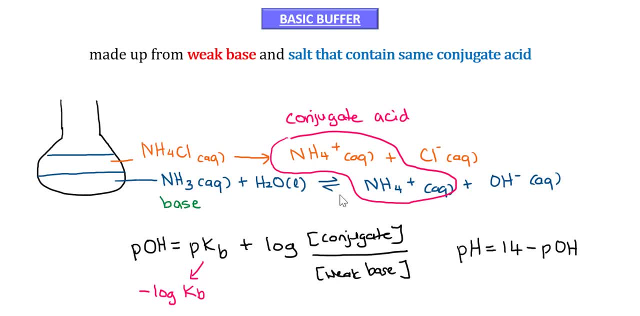 while the ammonia, which is a weak base, will slightly dissociate into the ammonium ion and the hydroxide ion. The ammonium ion that's present in both solutions is the same conjugate acid, So this solution is a buffer solution. 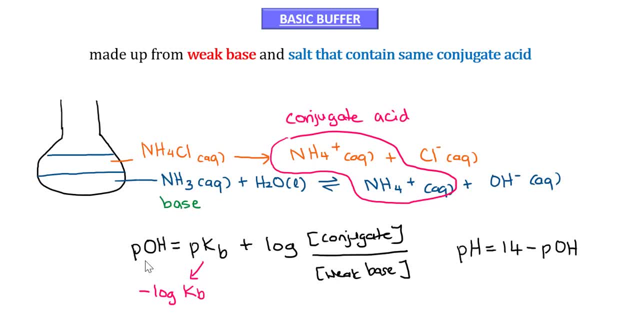 To find the pH of the basic buffer, we need to calculate the value of the pOH by using the Henderson-Hasselbalch equation, which is pKb plus log concentration of conjugate acid over the concentration of the weak base. The concentration of the conjugate acid is equal to the concentration of the salt. 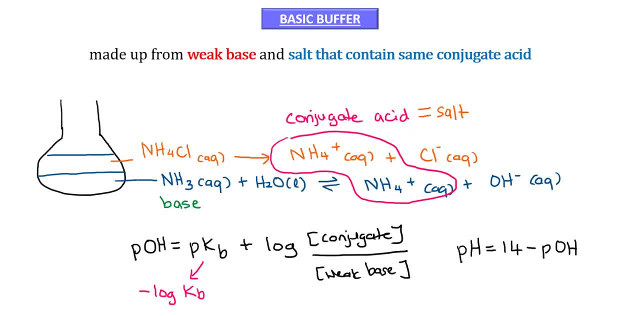 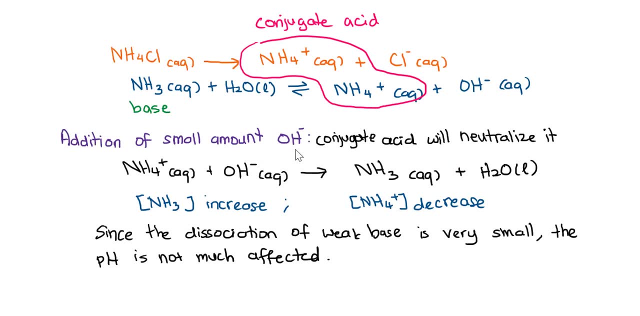 since the salt is fully dissociated and forms the conjugate acid ion. When a small amount of a strong base is added, the conjugate acid will neutralize it. So the conjugate acid will react with the base to form the ammonia and also water.